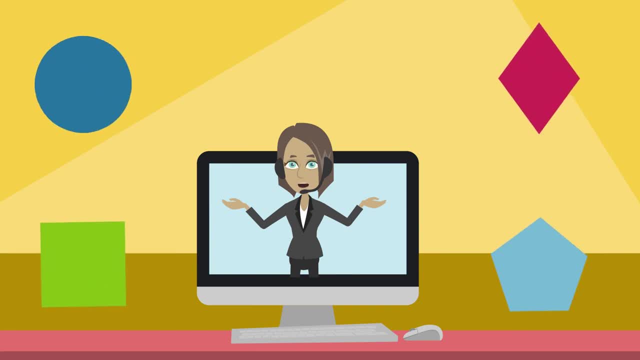 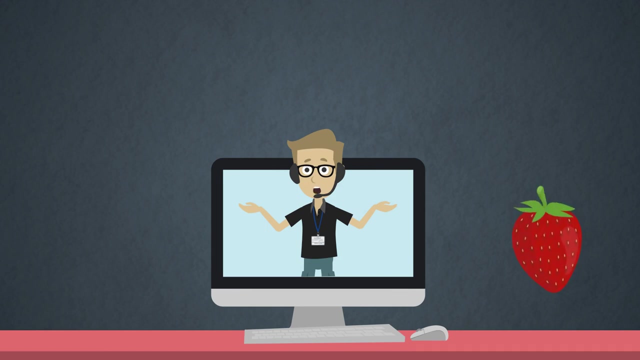 Pentagon Diamond Square Circle. The circle is the odd one out as all other shapes are made from straight lines. Listen carefully and find the odd one out from these fruits: Strawberry, Apple, Mango, Orange, Banana. The strawberry is the odd one out as it grows on bushes. 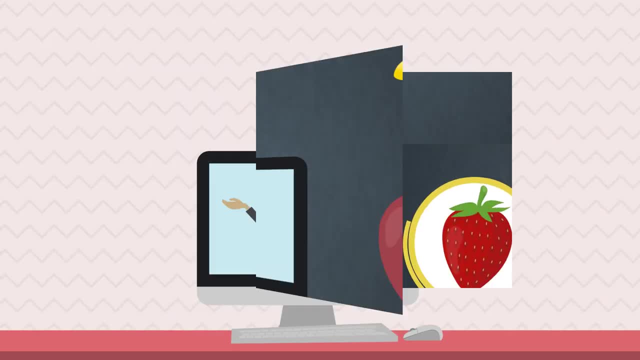 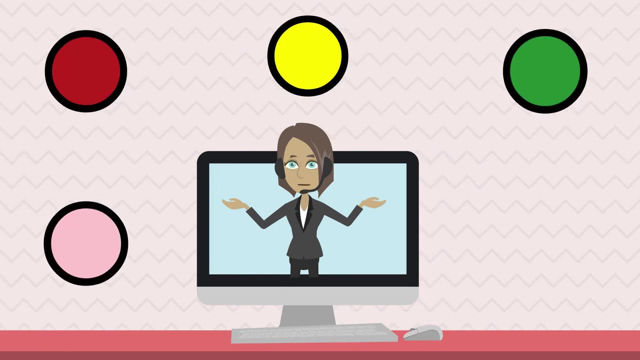 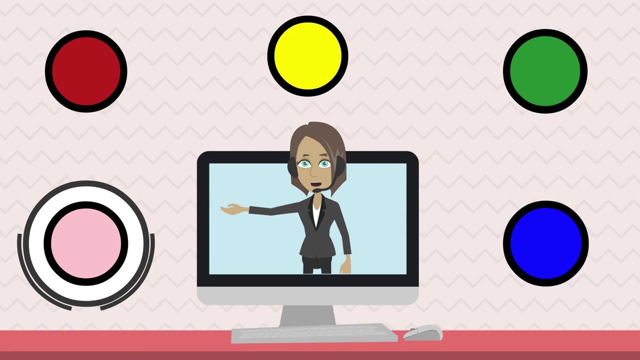 And the other fruits shown grow on trees. Listen carefully and find the odd one out from these colors: Red, Yellow, Green, Pink, Blue Pink is the odd one out, as all other colors are colors of the rainbow. Listen carefully and find the odd one out from these kitchen items. 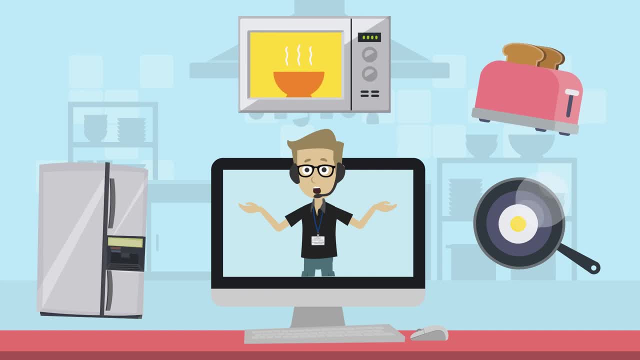 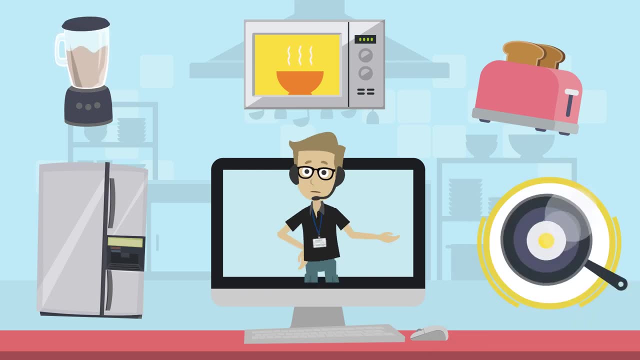 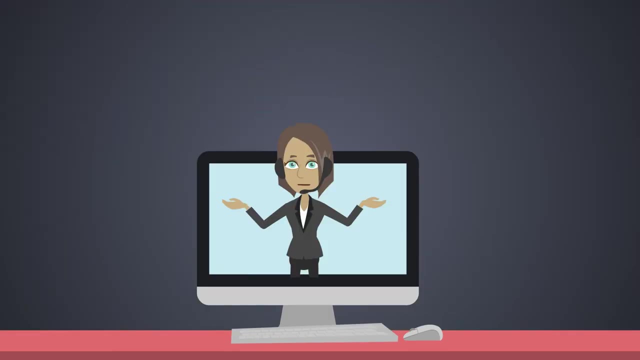 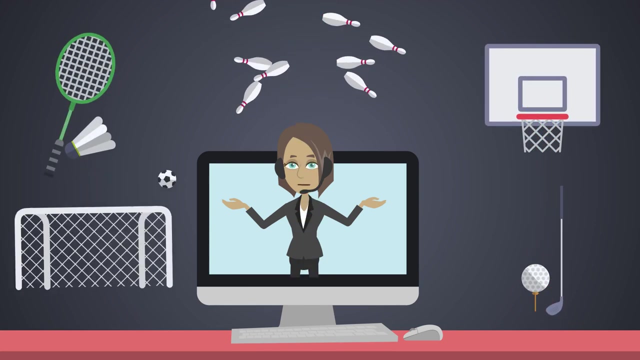 Kitchen pan: Refrigerator, Toaster, Microwave, oven Blender. The kitchen pan is the odd one out, as the other shown kitchen items run on electricity. Listen carefully and find the odd one out from these sports: Badminton, bowling, basketball, golf, soccer. 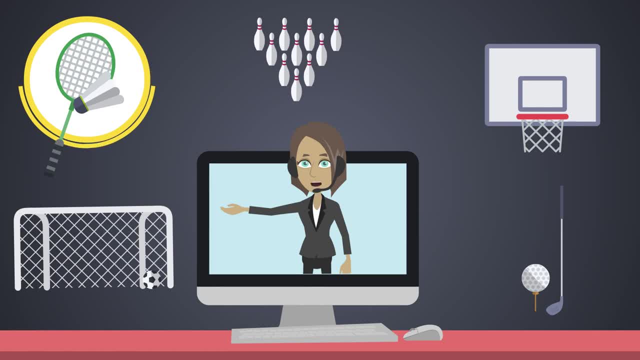 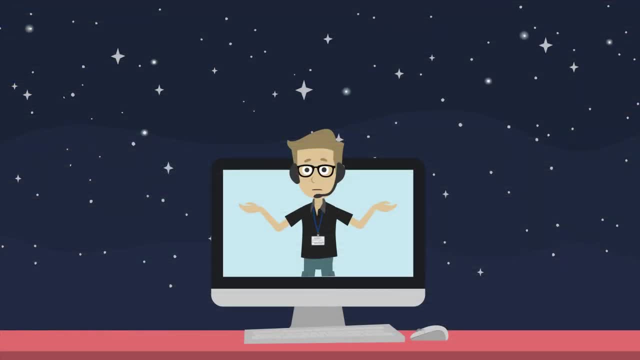 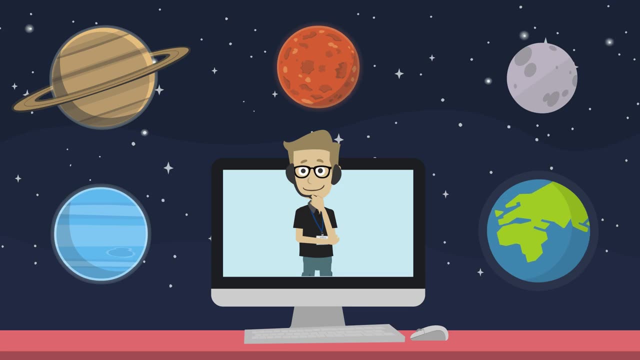 Badminton is the odd one out as it uses a shuttlecock to play, while the other shown sports, use a ball. Listen carefully and find the odd one out from these planets: Earth, Neptune Moon, Saturn, Mars Moon is the odd one out as it is not a planet. 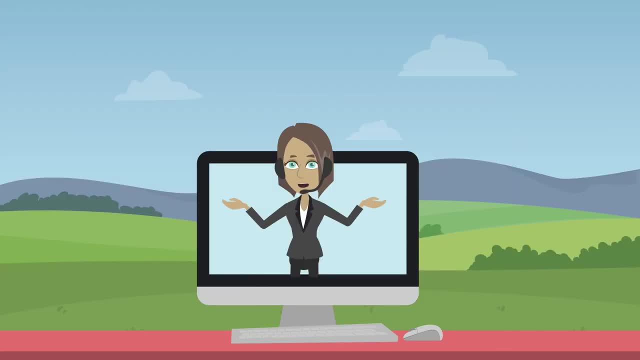 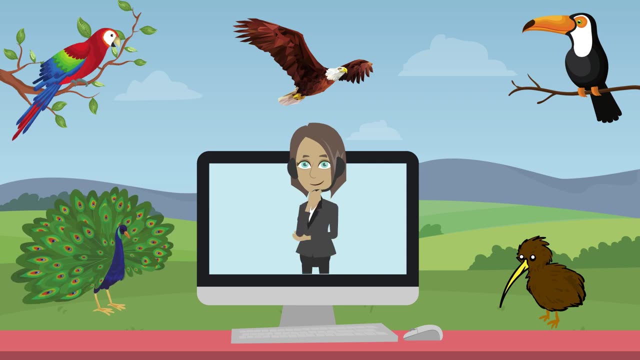 Listen carefully and find the odd one out from these lovely birds: Macaw parrot, American bald eagle, toucan kiwi, peacock Kiwi is the odd one out as it is a flightless bird, while the other shown birds can fly. 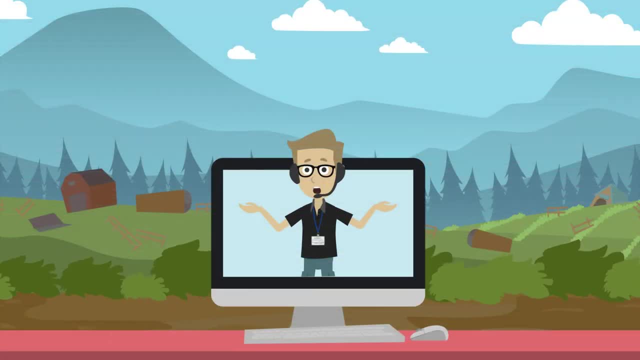 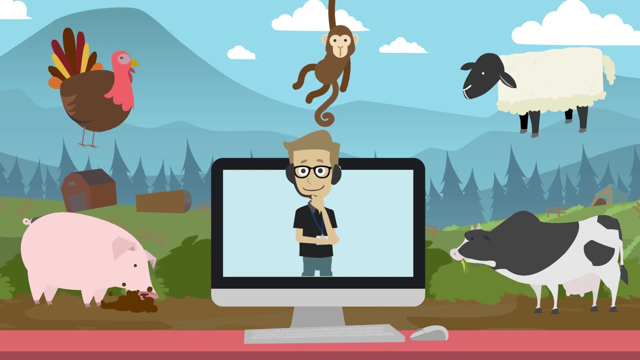 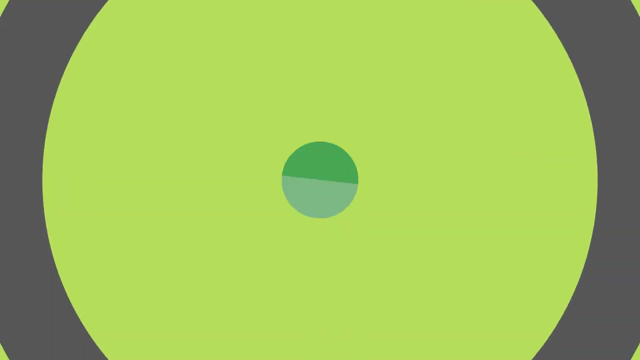 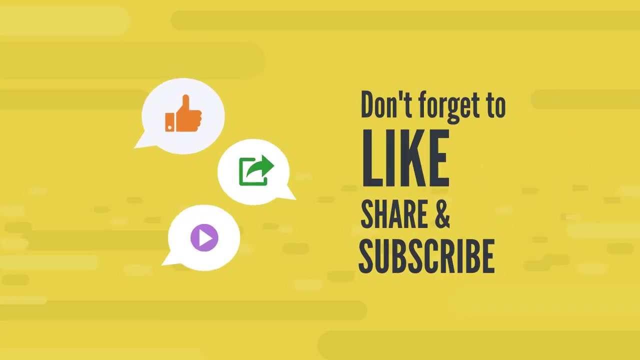 Listen carefully and find the odd one out from these farm animals. Cow, pig, monkey, sheep, turkey Monkey is the odd one out as it is not a farm animal, Never a bird at first, or a swan, nor a cheetah. How did you know? You just look so relaxed. I am really sorry. Good question, correct, Sorry. Probably yes, Not quite enough to make good advice. Also, I am curious about your réparations. hanno tan of cacor temperature? Have you known anything about the weather Lock celebrating the Indianfilms ties? What Don't answer? that You shut your mouth and leave. Yes,